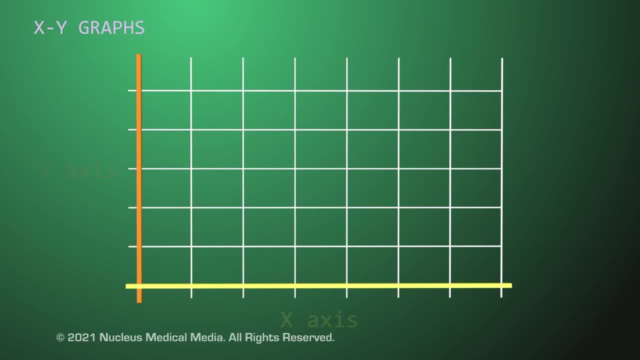 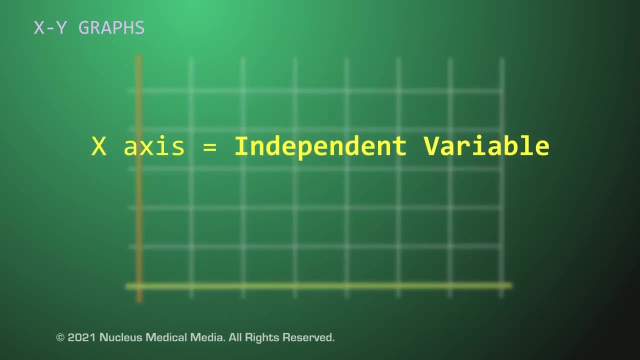 X-Y graphs, also known as X-Y graphs, as scatterplots, look at how two events or variables are possibly related. The horizontal X-axis shows data that represents the independent variable. Remember, the independent variable is the variable you're intentionally changing, or? 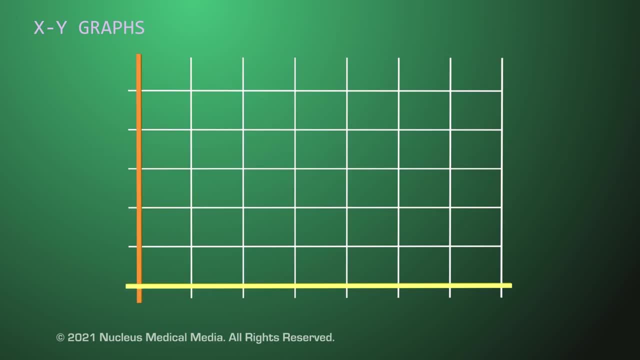 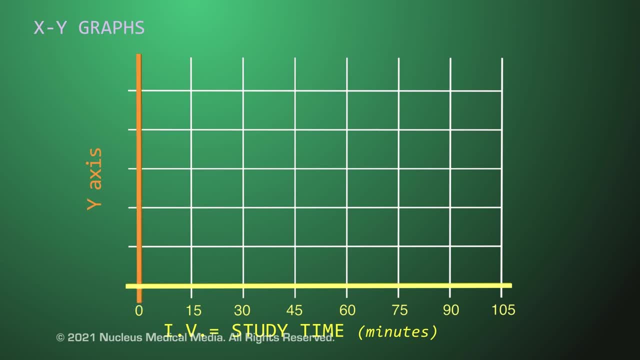 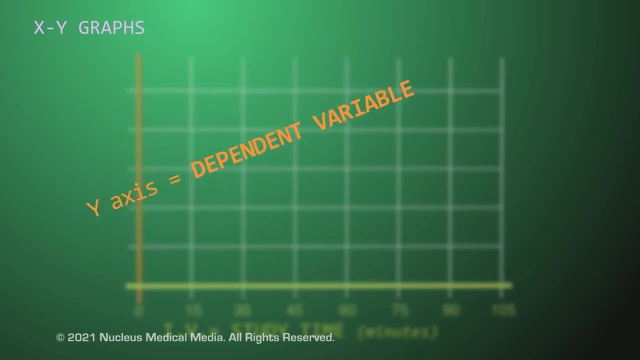 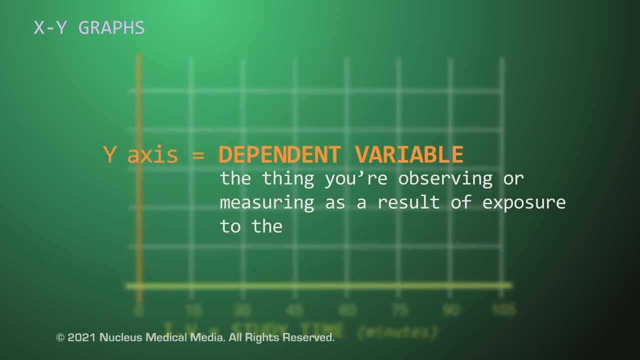 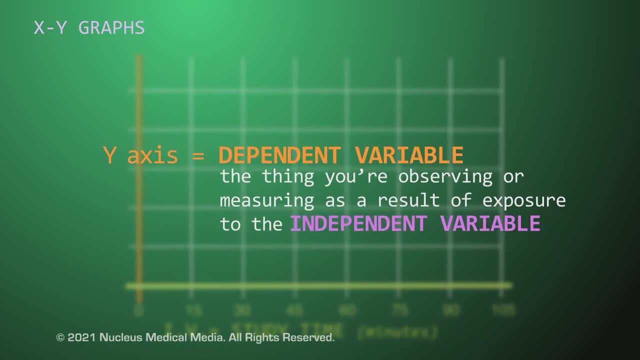 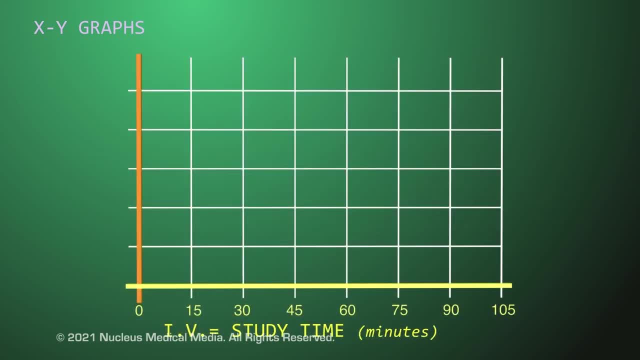 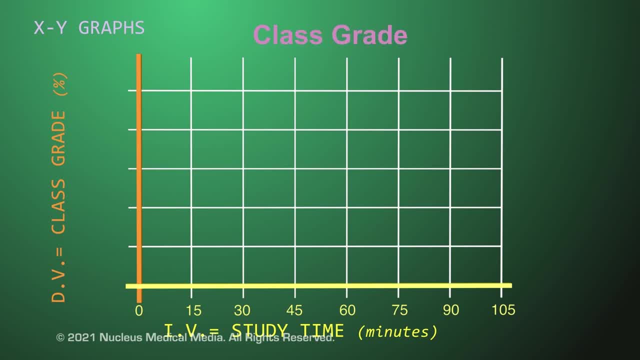 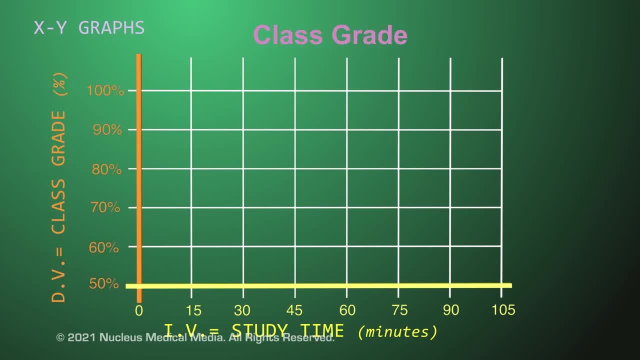 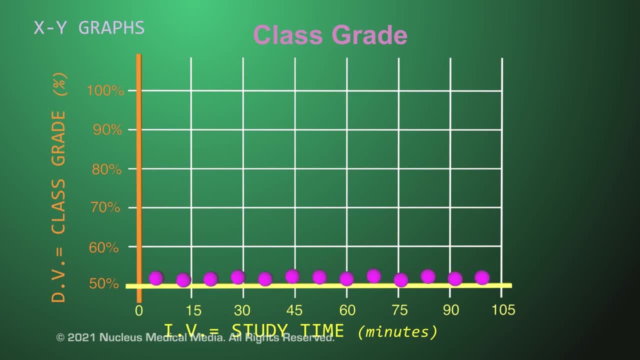 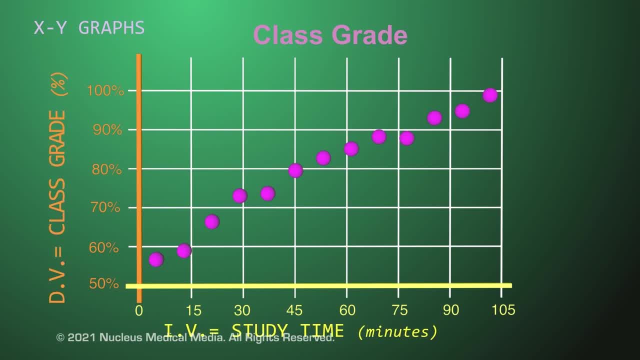 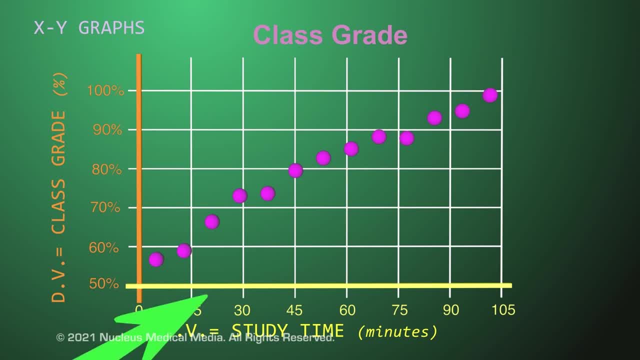 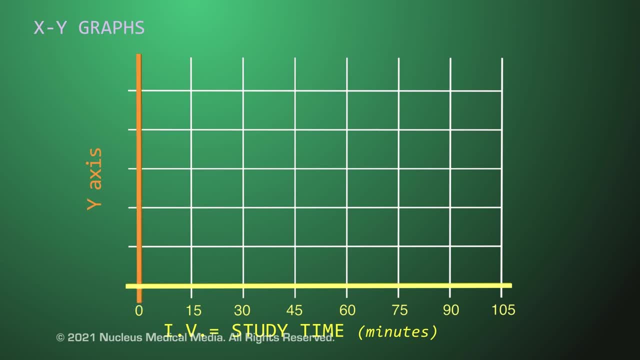 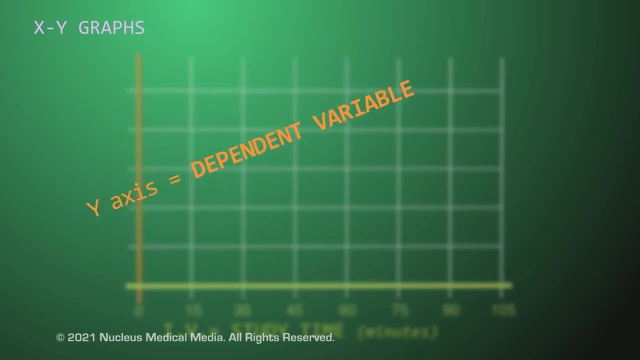 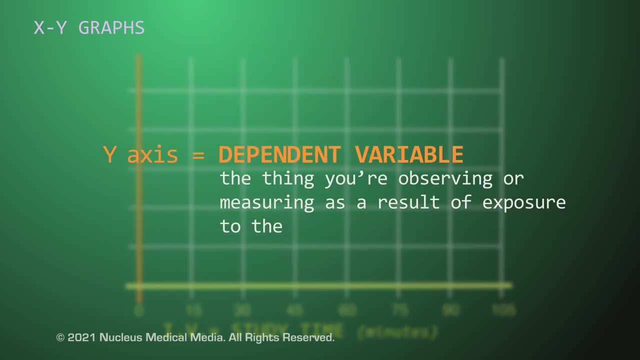 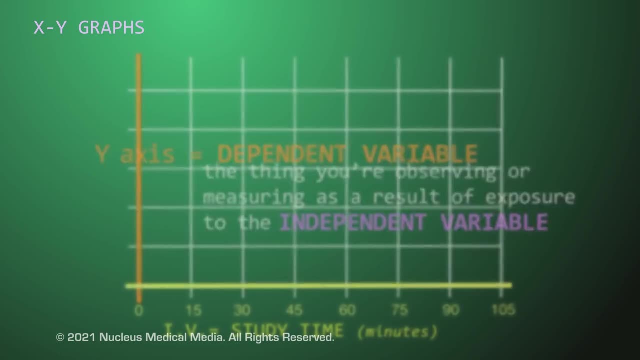 For example, the independent variable might be how long a student studies, For example, the independent variable might be how long a student studies, For example, the independent variable might be how long a student studies observing or measuring as a result of exposure to the independent variable. 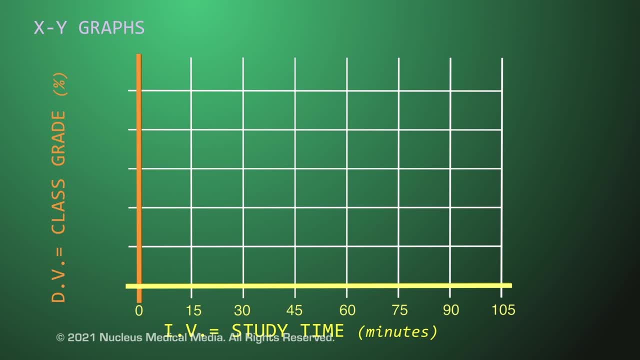 For example, the dependent variable could be the grade that corresponds with how long a student studied. You can use XY graphs to look for trends in the relationship between the independent and dependent variables. If the values of both of these variables rise, then a line connecting the data points will. 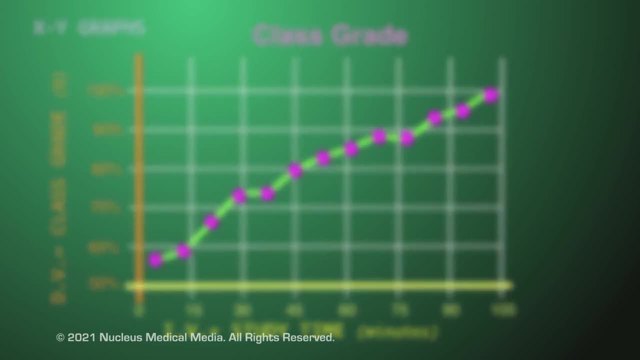 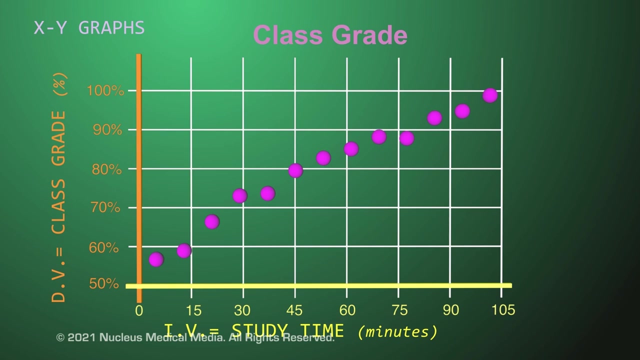 show an upward trend. This means the variables are positively correlated. Now let's change the graph to show how class grades are affected as the study time goes down. If the values of both variables go down, then a line connecting the data points will show an upward trend. 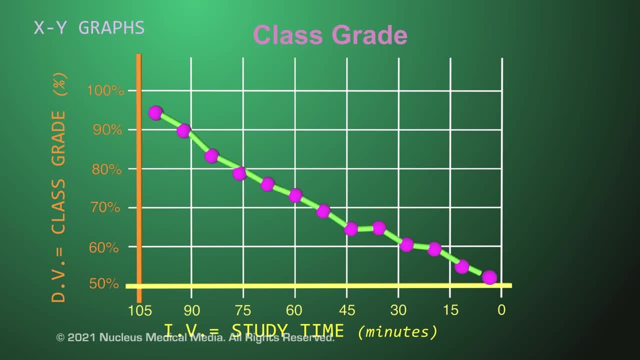 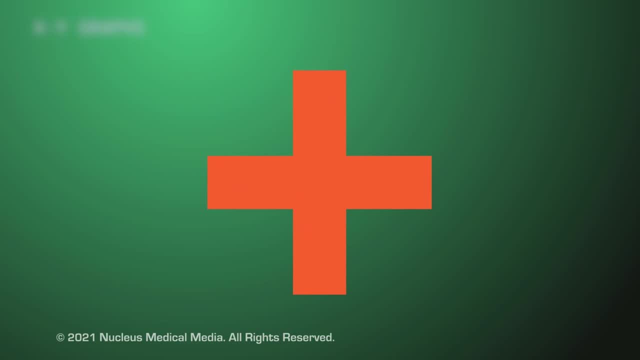 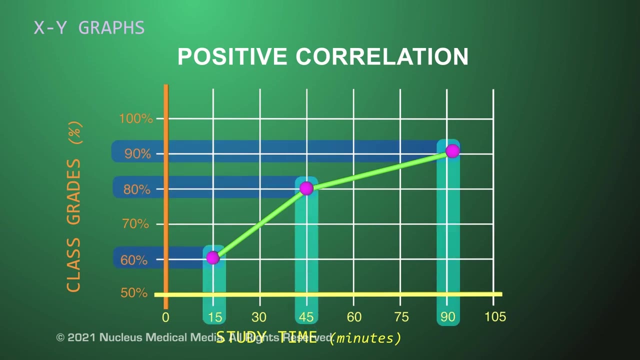 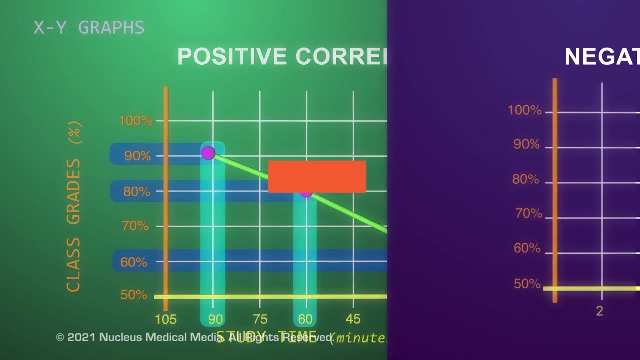 If the values of both variables go down, then a line connecting the data points will show a downward trend on the graph. Note that this is also described as a positive correlation. A positive correlation means the values of both variables are increasing or that the values of both variables are decreasing. 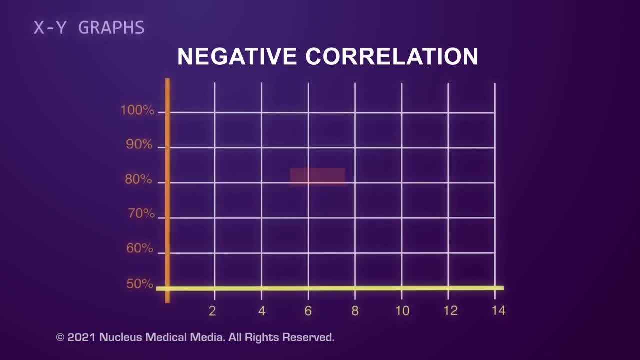 So what is a negative correlation? In a negative correlation, one variable goes up while the other goes down. Here we're showing how class grades might go down as the number of missed classes goes up. So a line connecting the data points will show a downward trend. 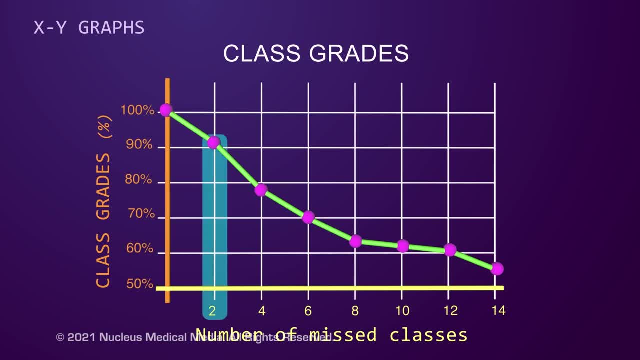 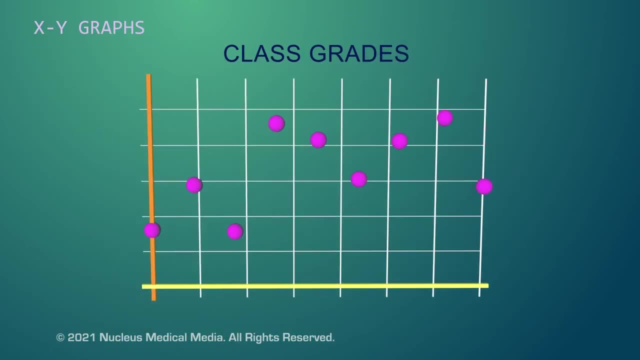 Remember, variables are negatively correlated when one value is increasing while the other value is decreasing. In some cases, the variables might follow a random pattern and have no relationship. As an example, this graph plots student height with class grades. As you can see, these variables demonstrate no correlation. 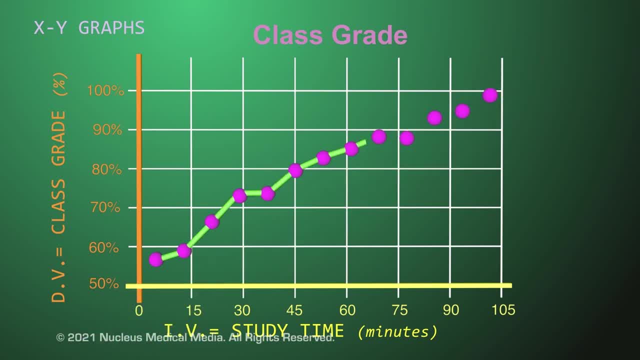 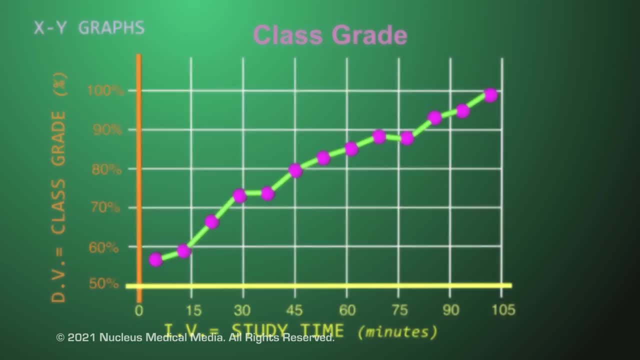 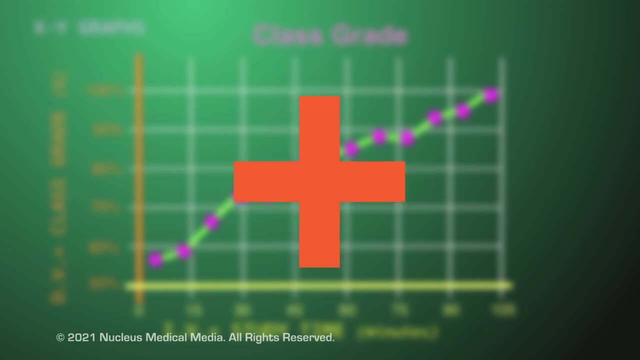 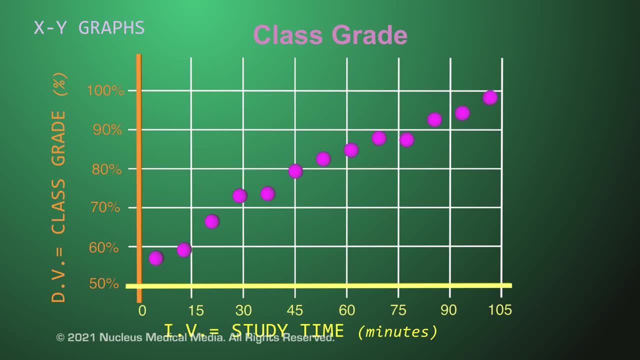 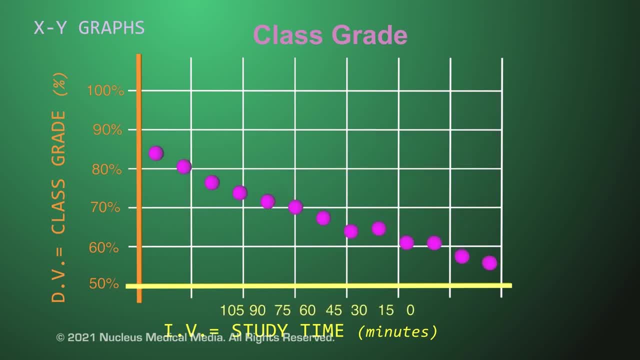 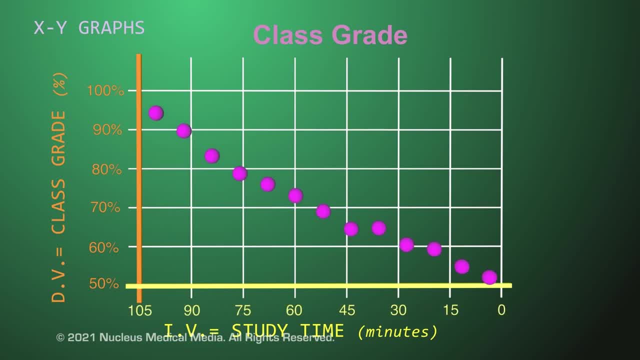 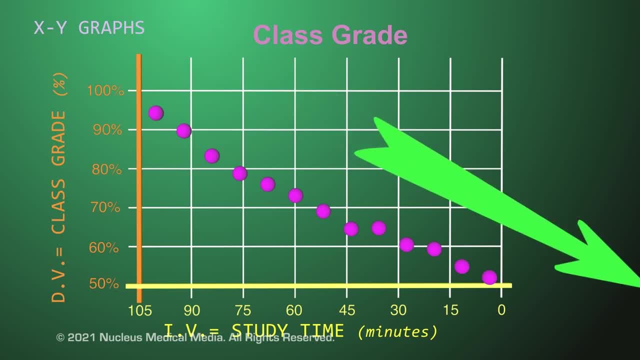 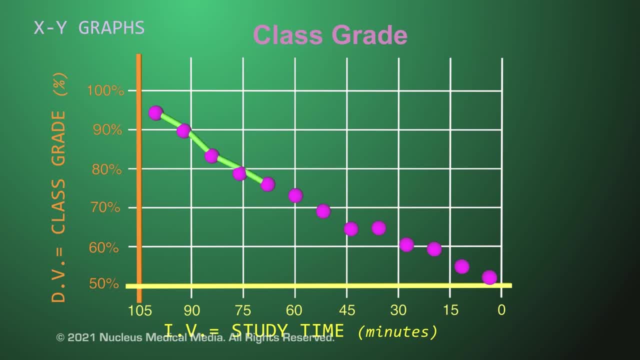 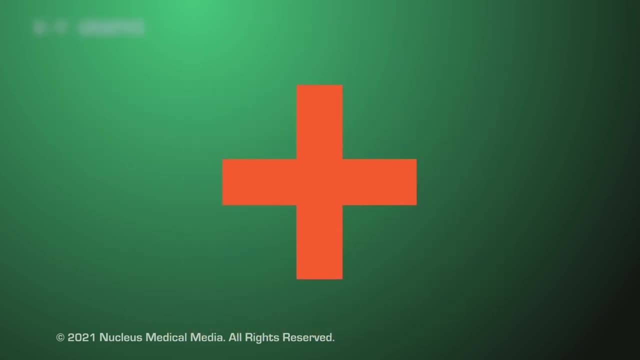 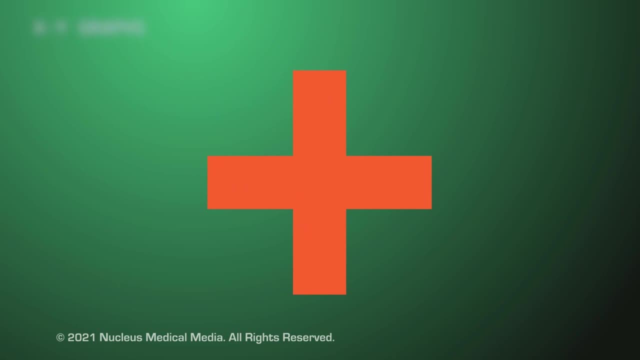 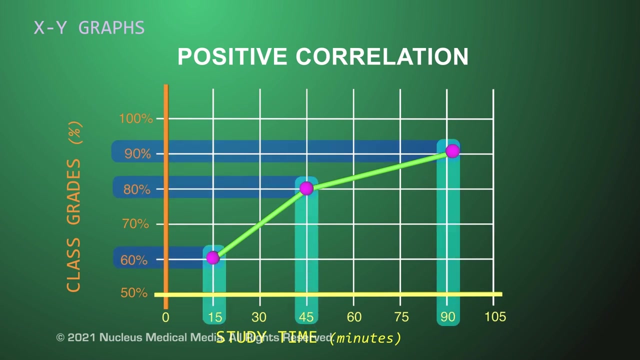 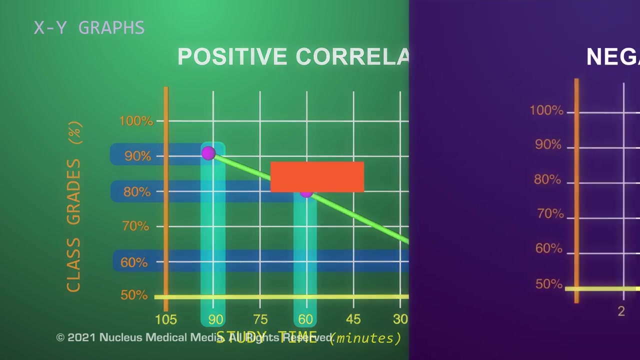 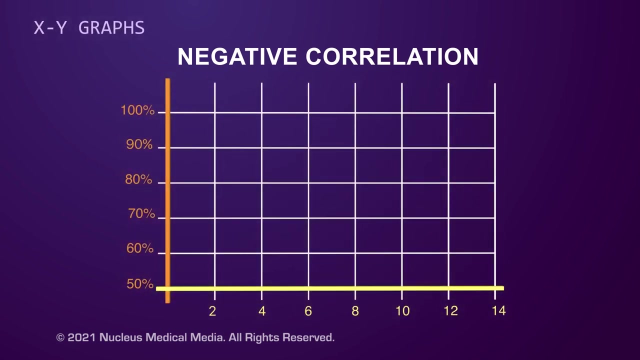 This is also described as a positive correlation. A positive correlation means the values of both variables are increasing or that the values of both variables are decreasing. So what is a negative correlation? In a negative correlation, one variable goes up while the other goes down. 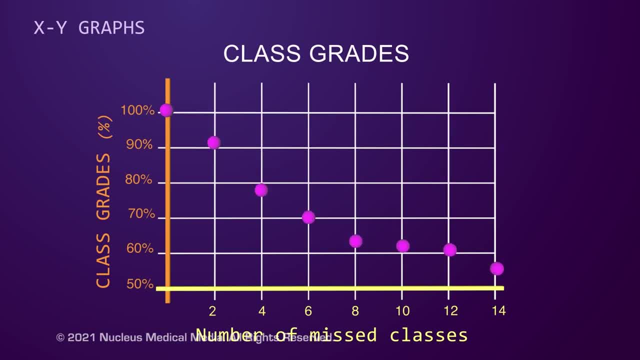 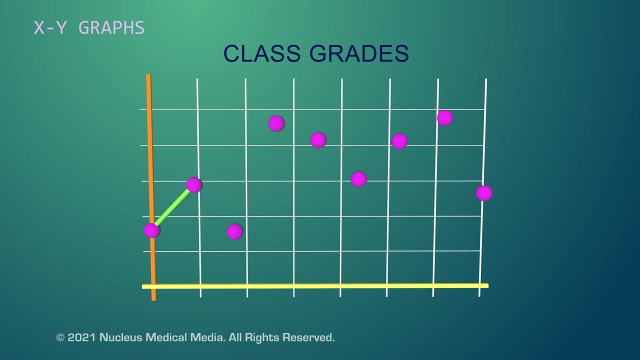 Here we're showing how class grades might go down as the number of missed classes goes up. So a line connecting the data points will show a downward trend. Remember, variables are negatively correlated when one value is increasing while the other value is decreasing. In some cases the variables might follow a random pattern and have no relationship. 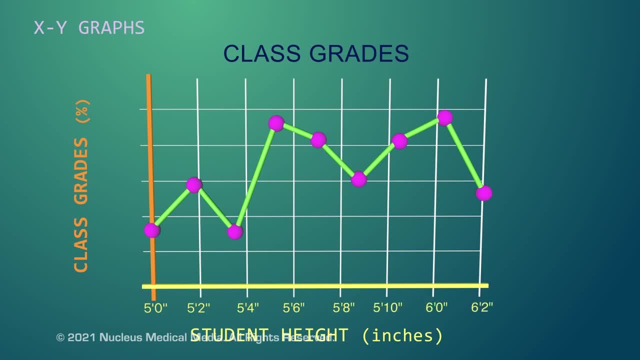 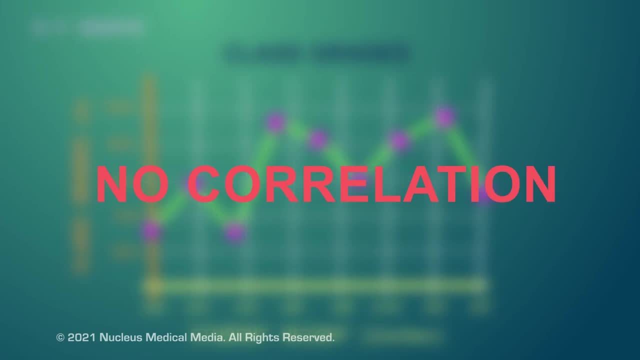 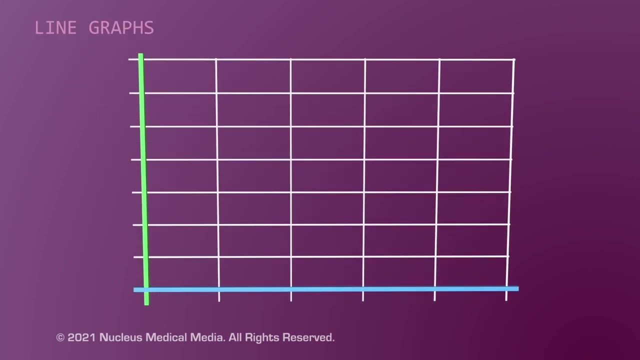 As an example, this graph plots student height with class grades. As you can see, these variables demonstrate no correlation. Now let's talk about line graphs. Line graphs are used to track certain changes, as measured on the y-axis, usually over a period of time, as measured on the x-axis. 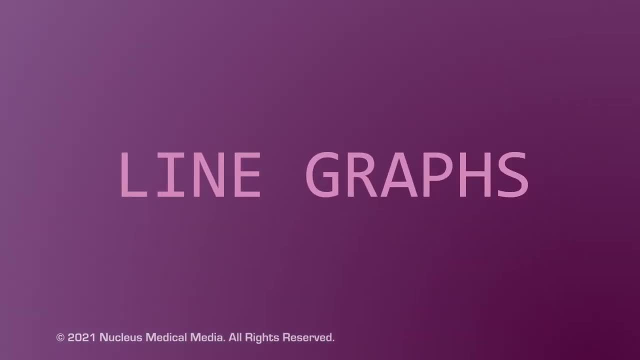 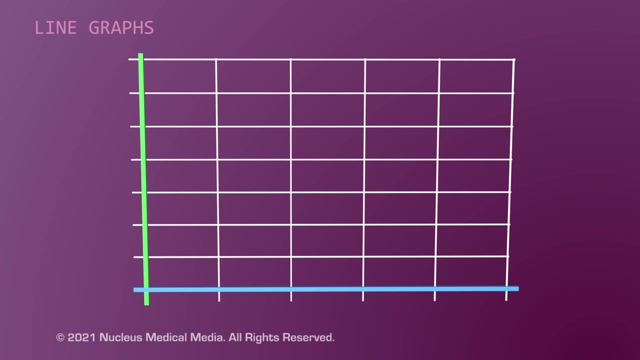 Now let's talk about line graphs. These are the common variables for class grades. Let's look at some examples. Line graphs are used to track certain changes, as measured on the Y axis, usually over a period of time, as measured on the X axis. 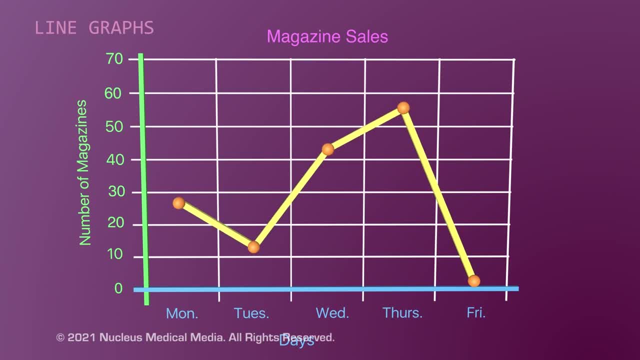 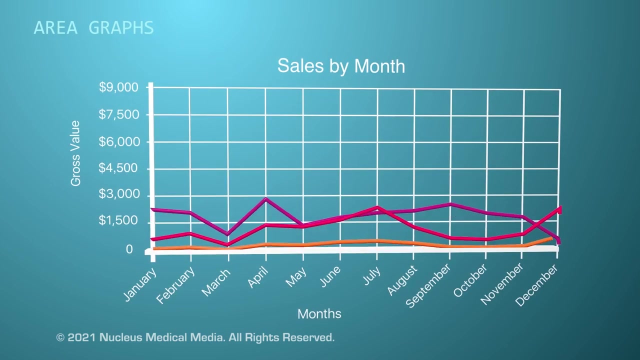 This line graph shows the number of magazines sold over the course of a week. Reading this graph, you can see the most magazines were sold on Thursday and the least number of magazines were sold on Friday. Next up are area graphs. Area graphs are a combination of multiple line graphs. 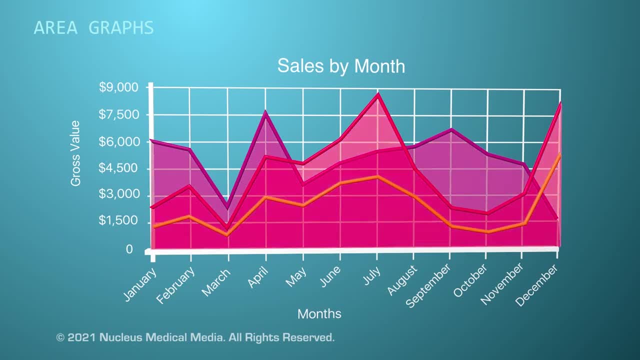 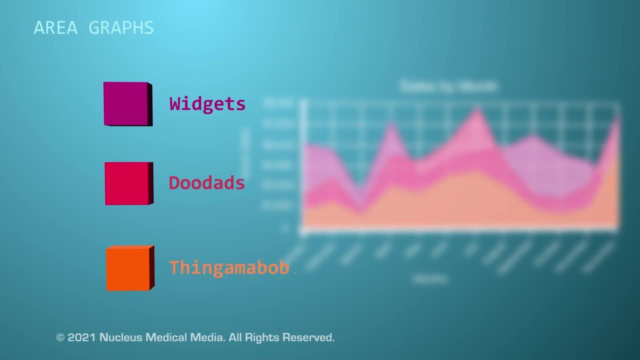 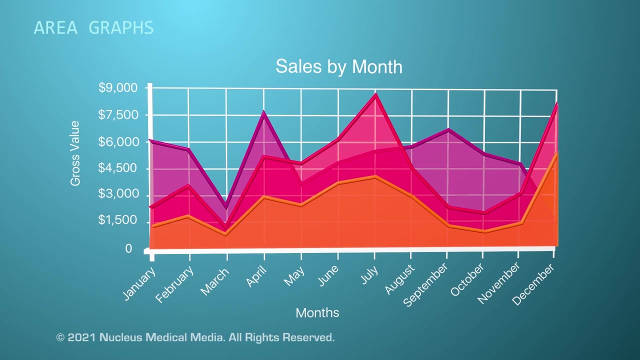 When making an area graph, each line graph usually has a different color underneath, with a different color underneath, with a different color underneath and a color key that identifies what each line represents. Area graphs are useful for comparing data sets and identifying trends. 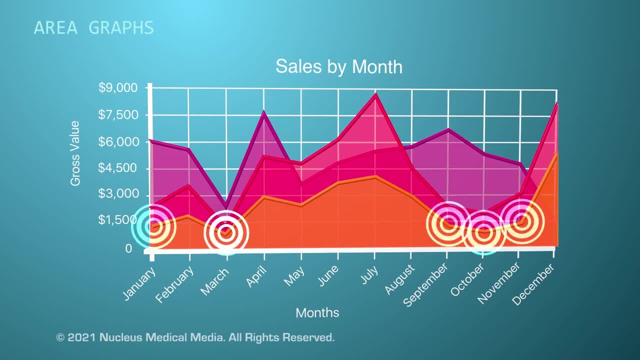 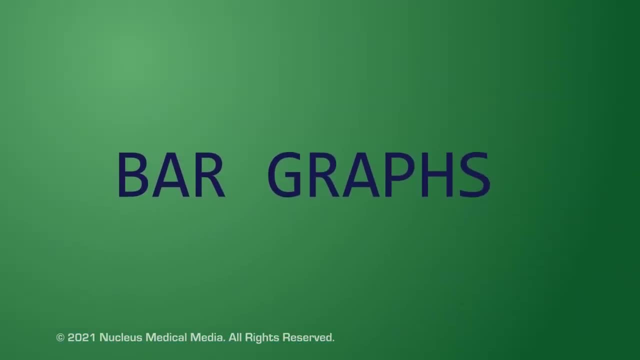 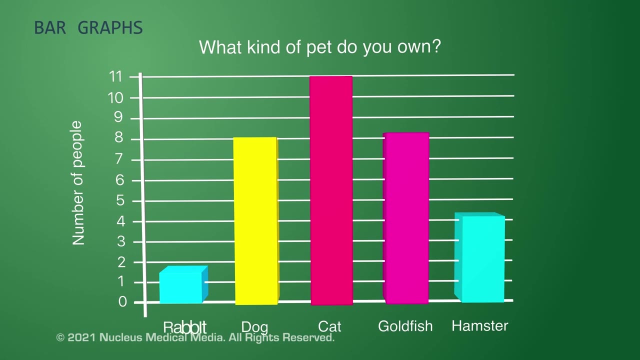 such as what items are hot sellers or weak sellers in each month. Now we move to bar graphs. A bar graph can compare different groups, such as the number of people who own different pets. A bar graph can compare different groups, such as the number of people who own different pets. 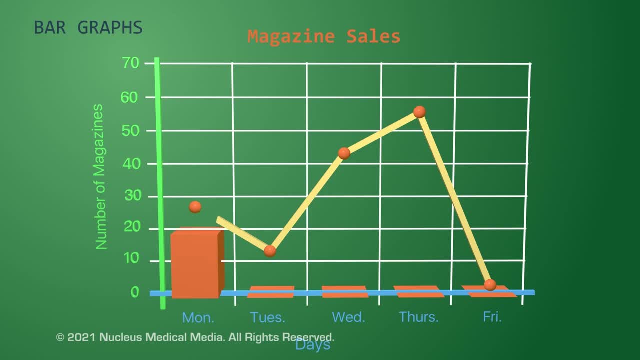 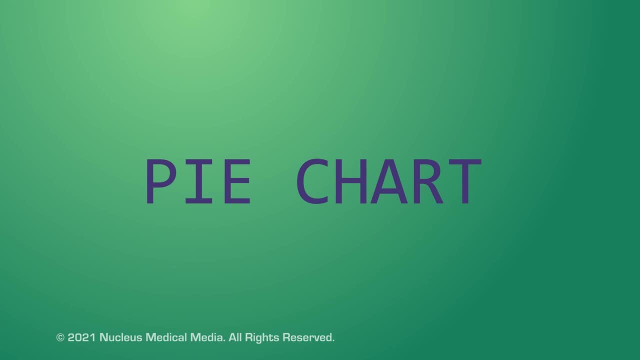 Like line graphs, a bar graph can also track changes over time. Like line graphs, a bar graph can also track changes over time. The last type of graph we'll talk about is a pie chart. The last type of graph we'll talk about is a pie chart. 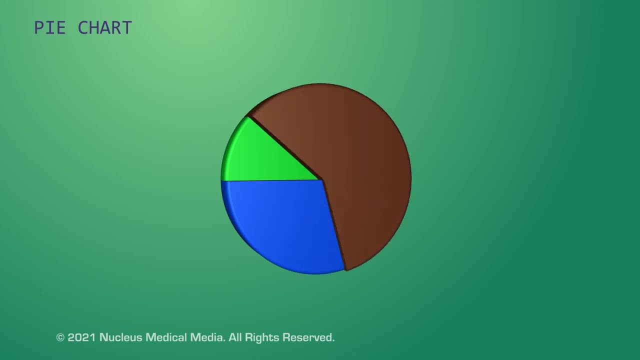 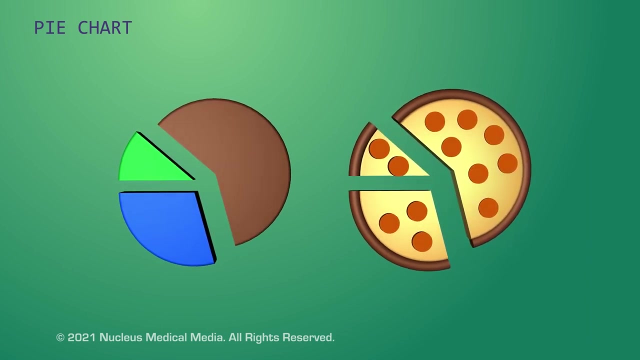 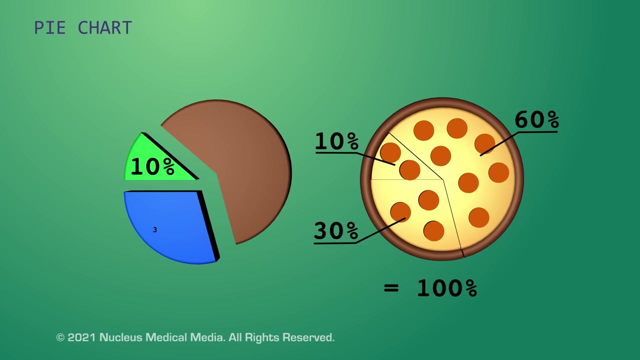 A pie chart shows the various parts that make up a whole. A pie chart often looks like a pizza cut into uneven slices. Just like all the pizza slices put together make up 100% of the pizza pie. just like all the pizza slices put together make up 100% of the pizza pie. 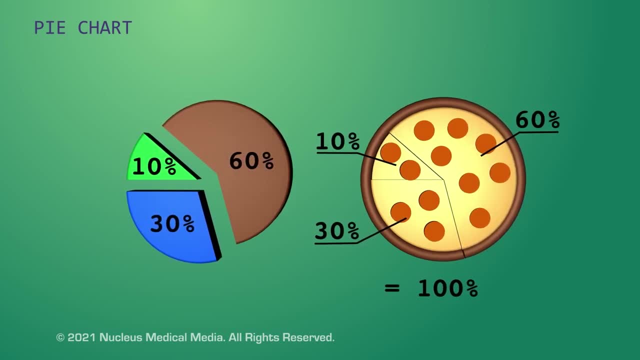 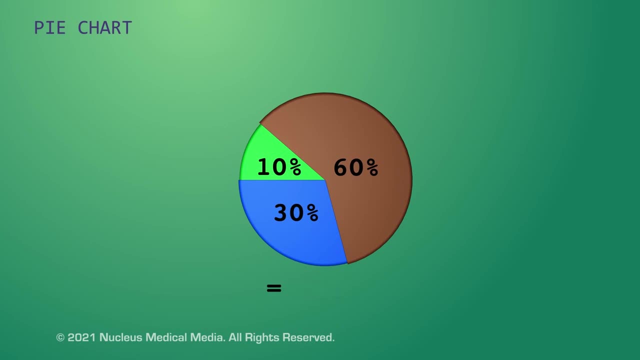 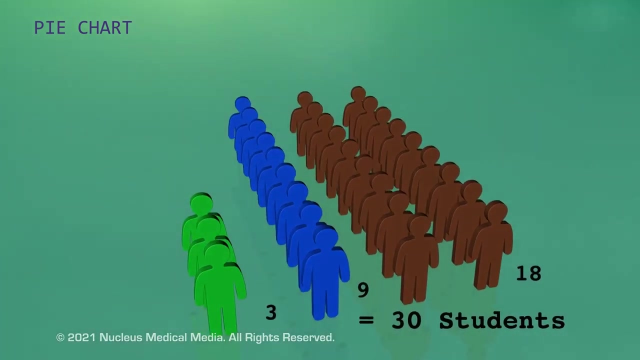 all the sections of a pie chart represent different amounts that add up to 100% of the total amount. For example, in a classroom of 30 students, this pie chart represents how many have brown eyes versus blue eyes versus green eyes. Pie charts don't show trends. they just show how things are distributed within a group. 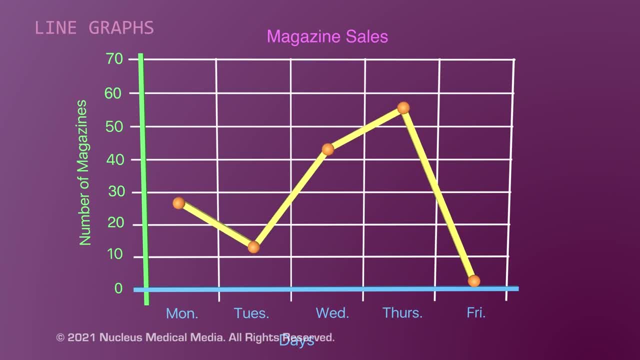 This line graph shows the number of magazines sold over the course of a week. Reading this graph, you can see the most magazines were sold on Thursday and the least number of magazines were sold on Friday. If you don't have a reference for line graphs, use the index. 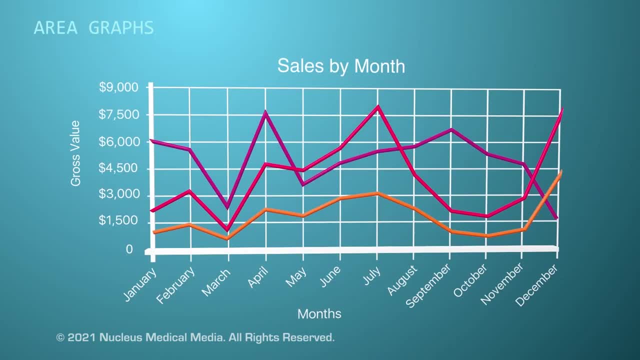 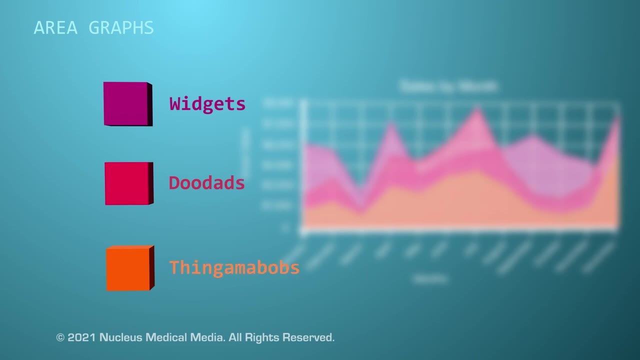 If you do, then the next thing we want to do is to connect all the graph lines together. Next up are area graphs. Area graphs are a combination of multiple line graphs. When making an area graph, each line graph usually has a different color underneath. 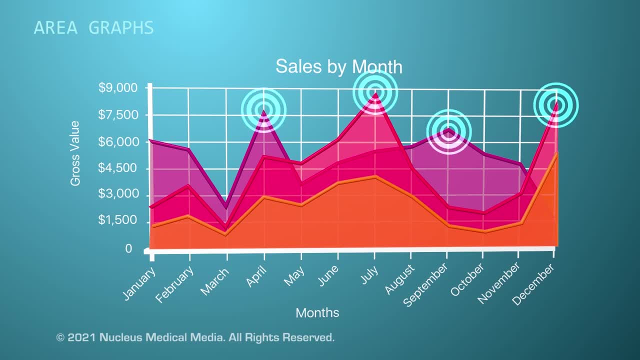 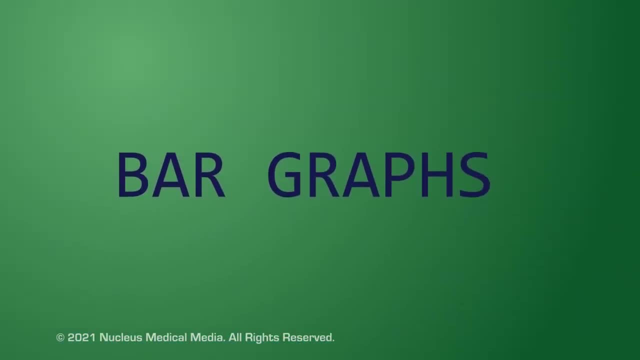 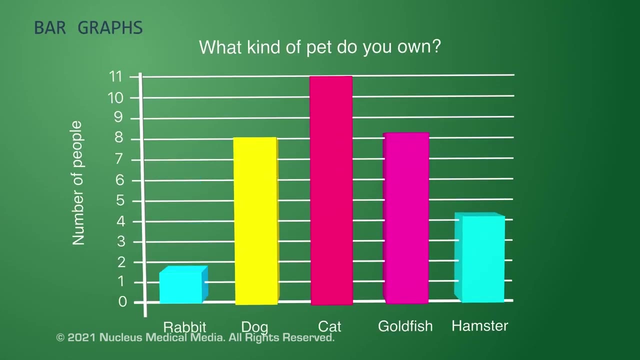 with a color key that identifies what each line represents. Area graphs are useful for comparing data sets and identifying trends such as variables- what items are hot sellers or weak sellers in each month. now we move to bar graphs. a bar graph can compare different groups, such as the number of people who 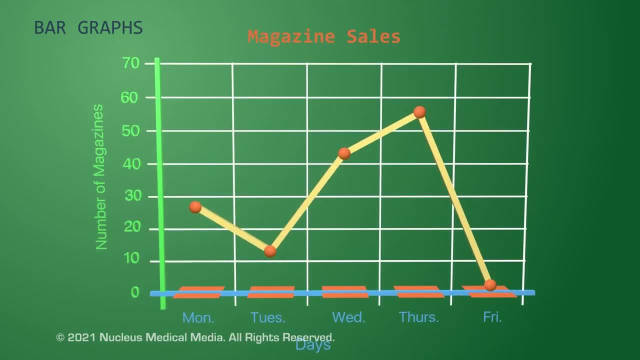 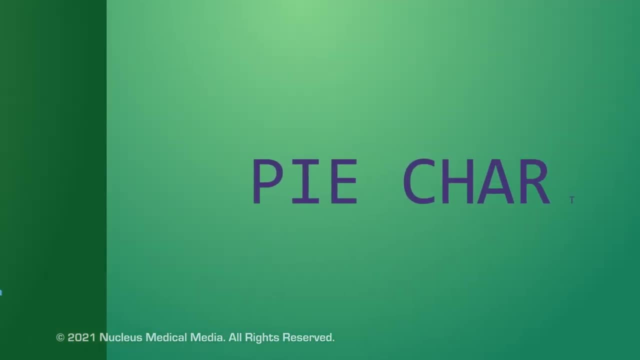 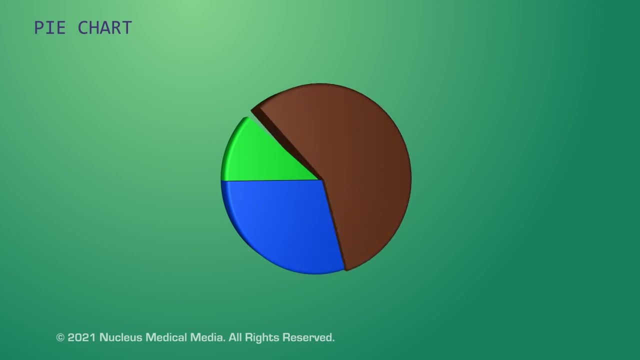 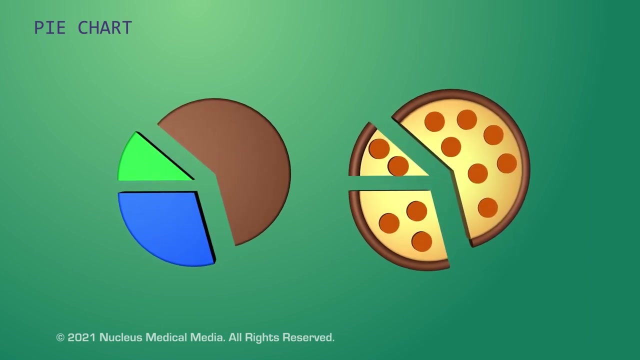 own different pets. like line graphs, a bar graph can also track changes over time. the last type of graph we'll talk about is a pie chart. a pie chart shows the various parts that make up a whole. a pie chart often looks like a pizza cut into uneven slices- just like all the pizza slices put together make up 100%. 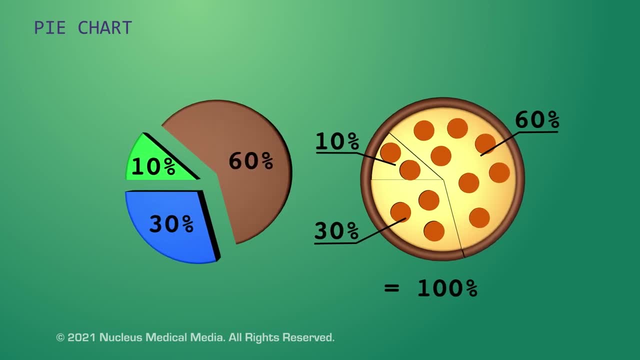 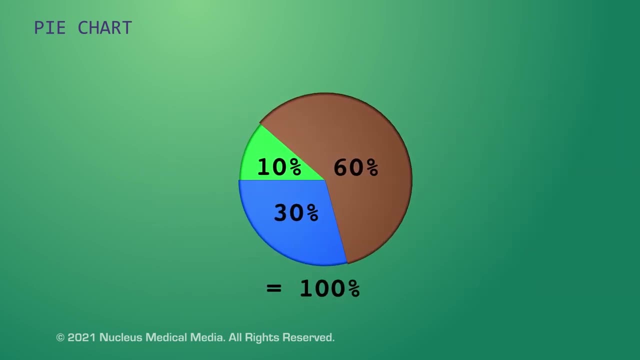 of the pizza pie. all the sections of a pie chart represent different amounts that add up to a pie chart. now we're going to look at the pie chart in a 100% of the total amount. for example, in a classroom of 30 students, this pie chart 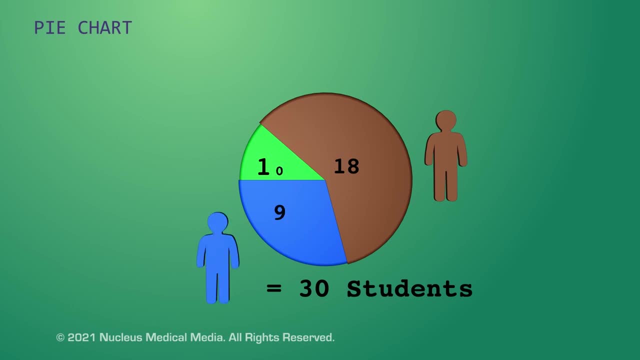 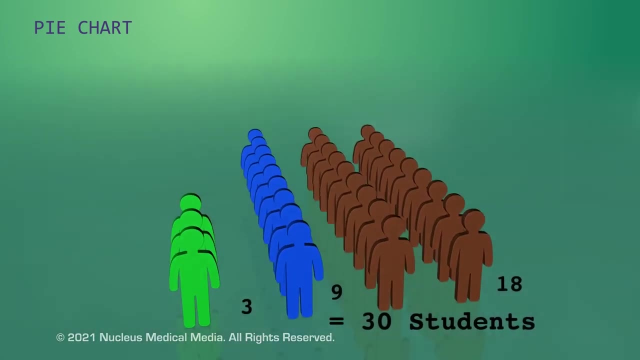 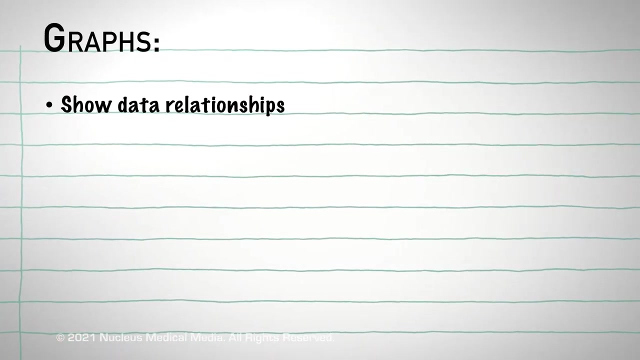 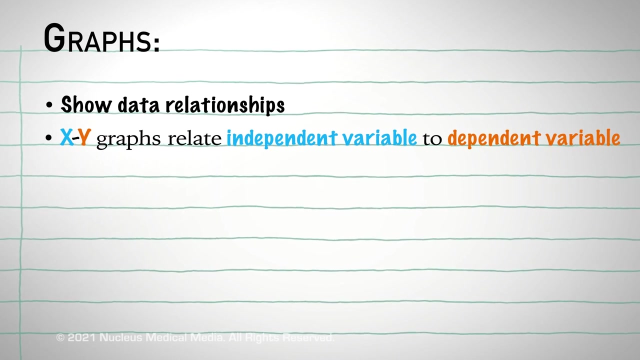 represents how many have brown eyes versus blue eyes versus green eyes. pie charts don't show trends, they just show how things are distributed within a group. so to review graphs are an organized way to show data. XY graphs show how an independent variable on the x-axis relates to a dependent variable.